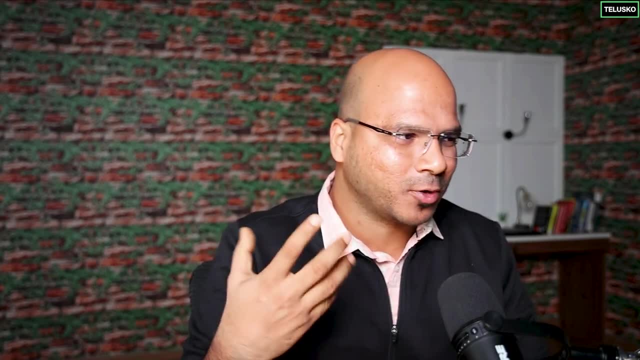 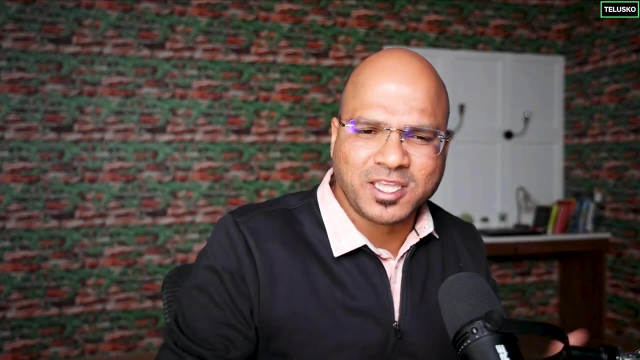 from now. it's also about thinking okay. So it's not just about coding something. Even when you start making something in your mind, you have to treat it everything as an object. example: let's say, if you want to add two numbers, the first thing you should 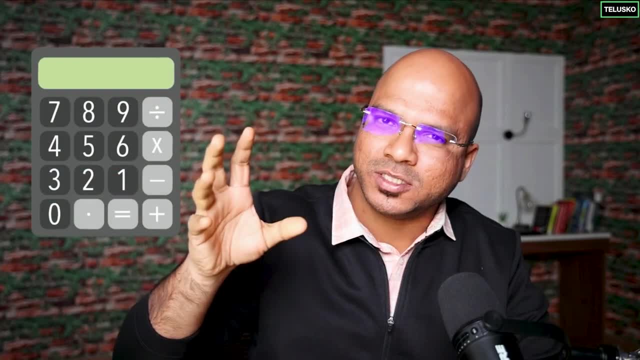 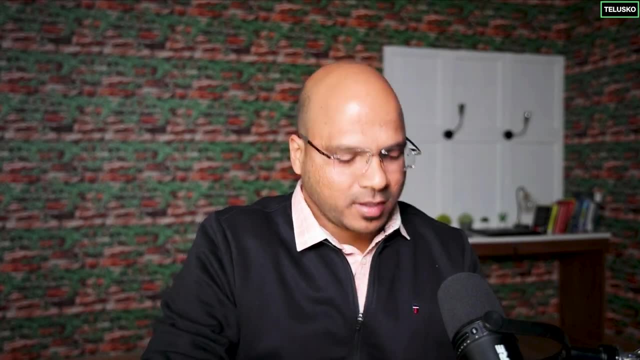 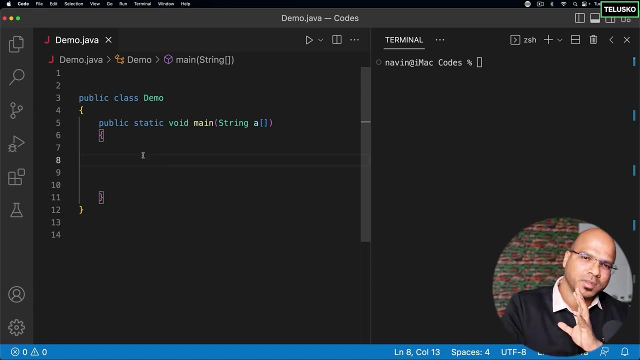 which should come to your mind is: okay, i need an object which can add two numbers. i'm getting my point right. everything you have to think in object way. so if you come back to programming, if you look at this example, of course we don't have an object here in this code, but you have to remember whatever. 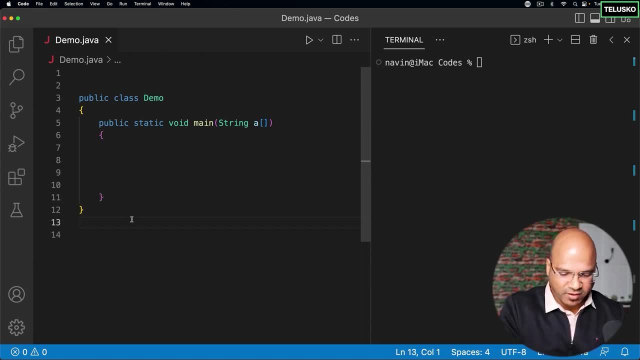 you want to do, you have to do with the help of object. so what we have discussed till now is there's a concept of object oriented programming. so basically, we have certain things here. we have a concept of object and this object will have a property and this will have behavior. so every 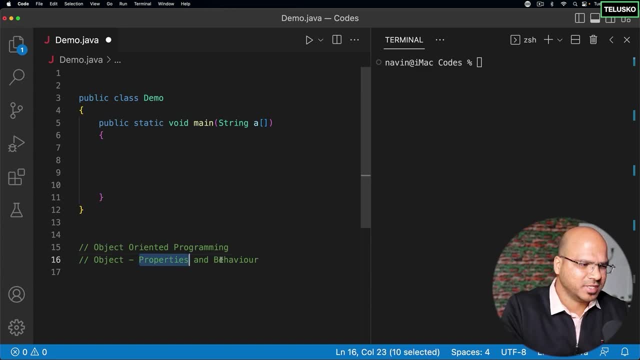 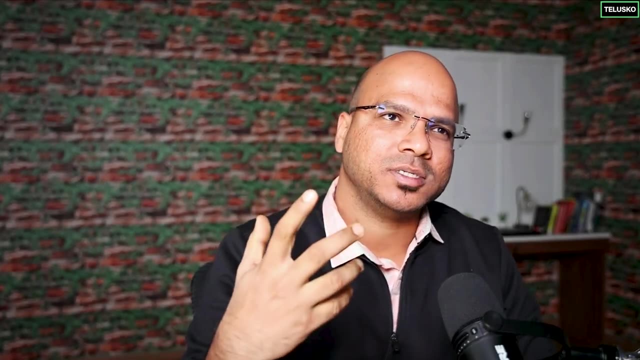 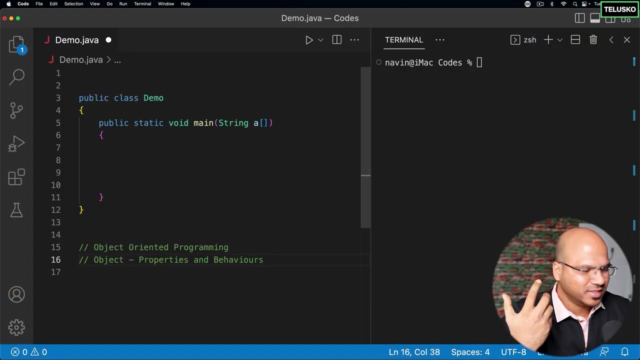 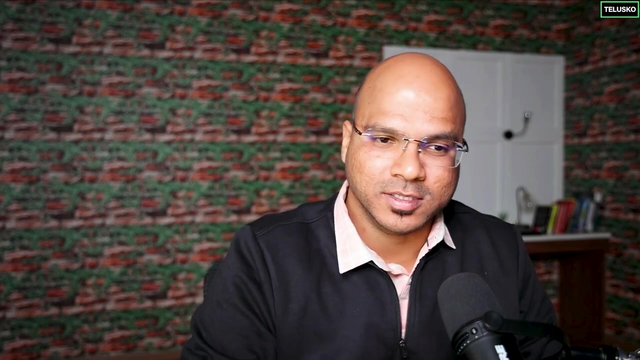 object will have a property and they also have a behavior. the properties can be multiple properties and multiple behaviors. example: let's say if i, as a human, if i'm an object, i know something, i know a to type code right and i behave based on what i know, so i can dance because i know how to dance. 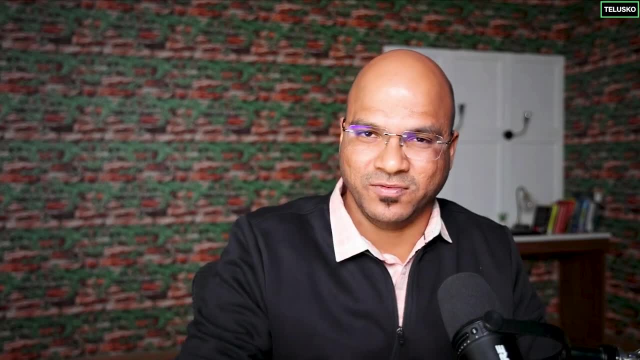 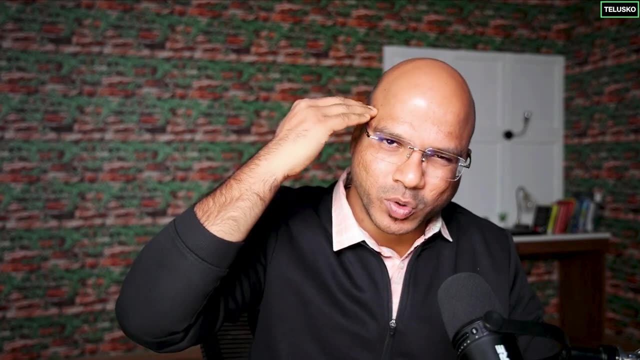 so that's your property. but you know how to dance. that's a behavior when you're dancing, when you're talking, when you're walking right. so i know my age as well. i know a lot of different. so whatever i know here is properties. what i, what i do, is behaviors. okay, but how do we create objects? 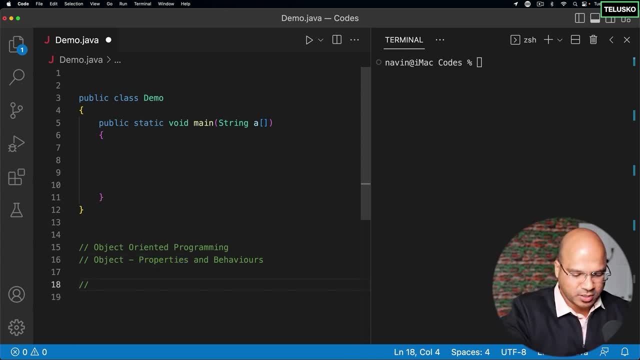 so in in java, if you want to get an object, we have to first create a class. okay, now why we need object and clause concept. so first of all, we have talked about object. everything has to be done with the help of object. in real life, we can't do anything without objects, so that's how it works. 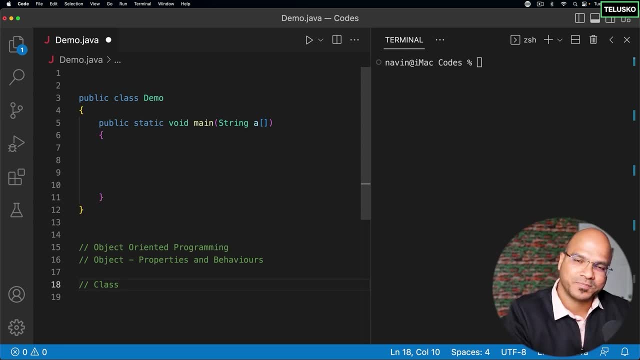 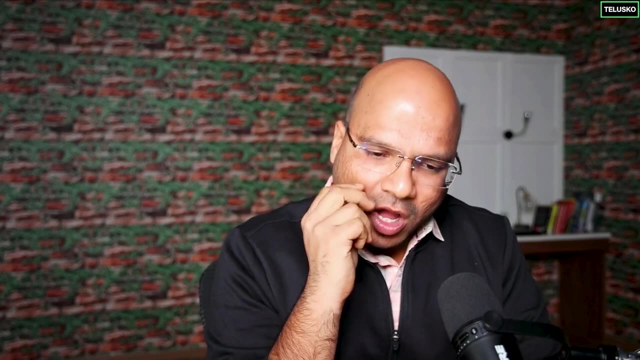 so in java as well. if you want to do something, you have to get an object. but how will you get an object and who creates this object? so let's talk about it now. if we talk about the concept of object, who create object in real world example? let's say, if we talk about this table, but i'm with 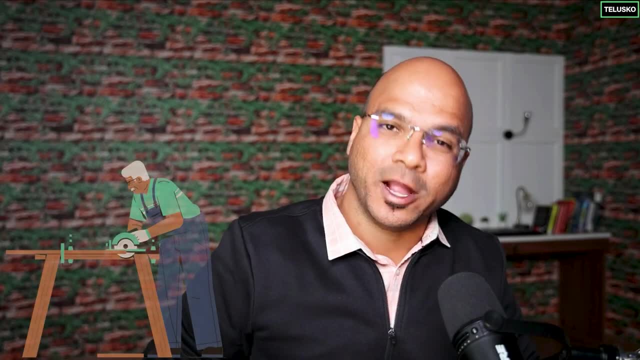 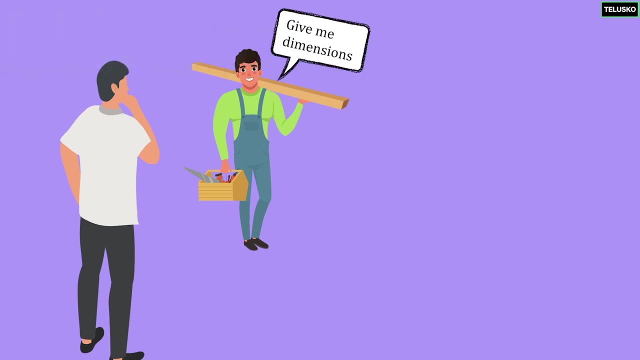 will have my systems. now this table is created by a carpenter. okay, so when you go to a carpenter by saying hey, i want a table, carpenter will say: okay, uh, i will give you a table, but tell me the exact dimensions. okay, uh, maybe take the carpenter, the actual guy who is making this table. he's very 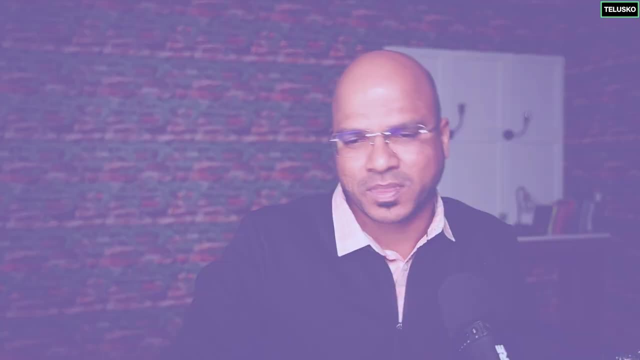 technical, so we have to explain in technical details and that's why we have some person in between who says: okay, you give me the details. okay, i will forward it to the person who says: okay, you give me the details. okay, i will forward it to the person who says: okay, you give me the details. okay, i will forward it to the. 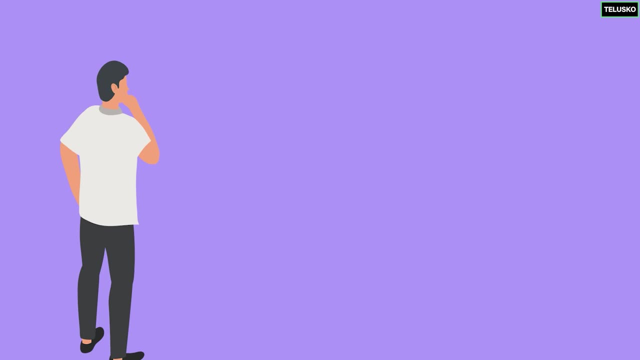 carpenter. so basically you give the details to the to that person, third person- and then that third person gives a detail to the carpenter. because carpenter understands on technical details and you understand only lay terms. i can say: hey, i want a table where i can keep my computer, where i can 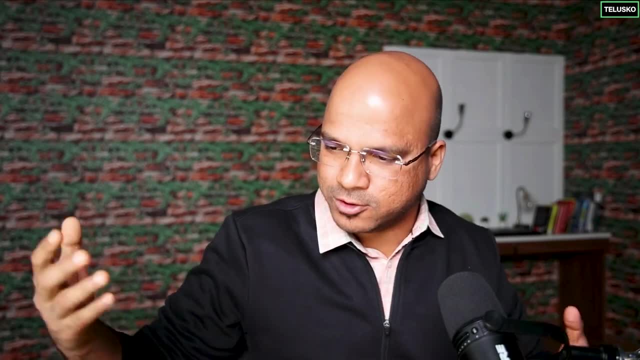 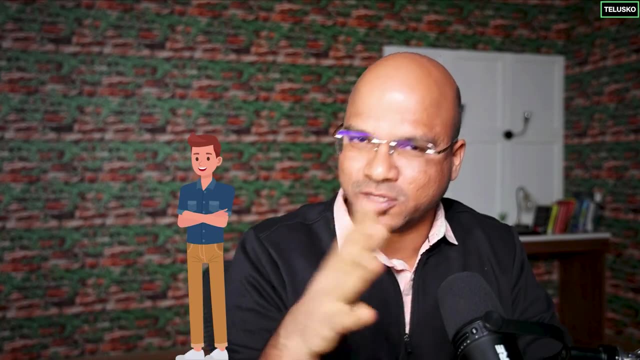 keep my monitors, my keyboard, mouse, uh, mobile phone and all the, all the different things which i have on the on the table here. so that person in the middle person will explain everything to a technique: the carpenter. okay, that's the dimension of a table, and then you can say, okay, i want a table, so i can. 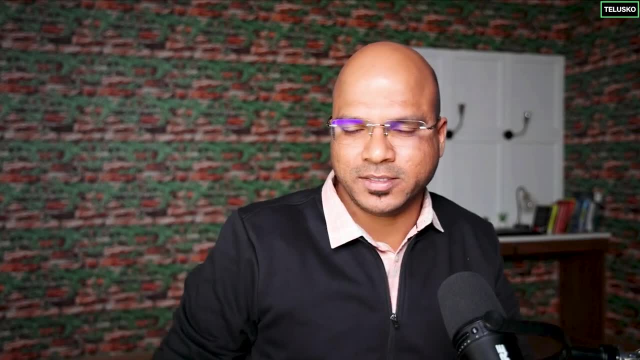 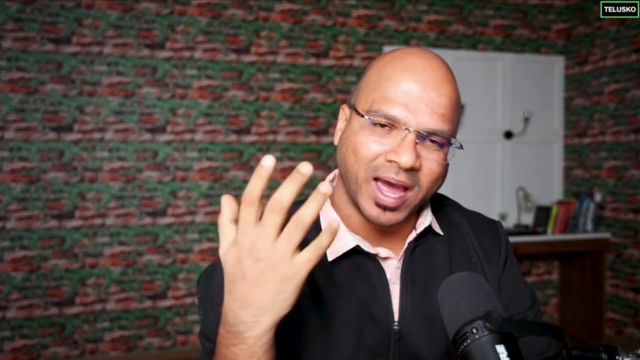 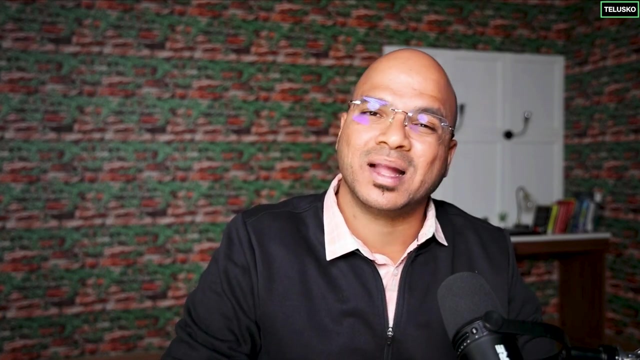 a person wants. this is the height which i want. based on my height, i want this table to be, and so all the details right, so got the point. so how do you give that design? so as a normal person, you give a design in a particular way and in programming you can give that design in a class file, so you 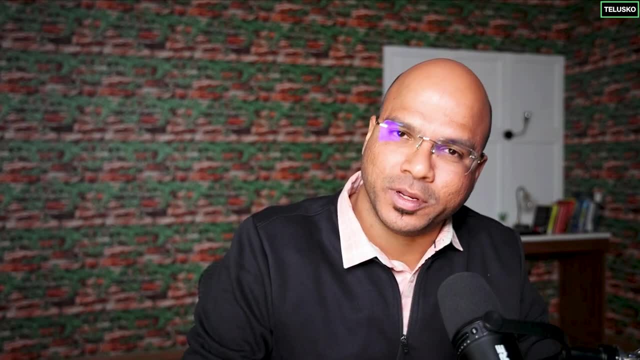 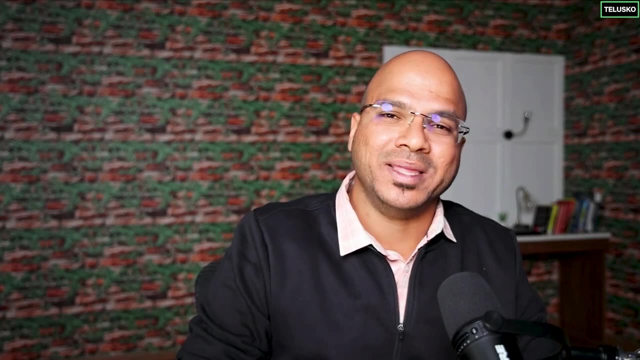 have to create a class file which will act as a blueprint for the carpenter or for the, for the, for the sum, for someone who can create object for you in java. now, who creates objects in java? it is your jvm. again, what is jvm? what is jre will have a digital discussion there, but at this point, 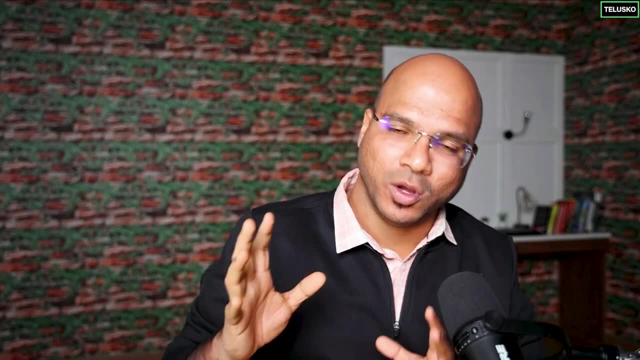 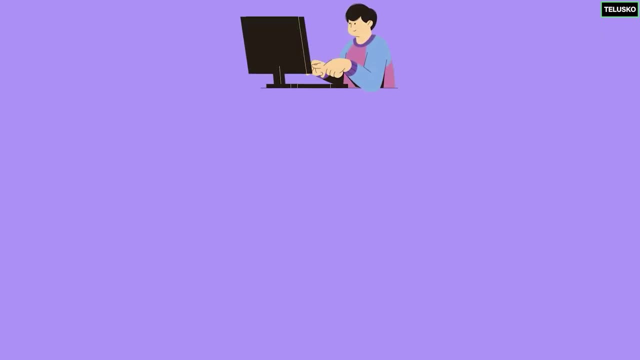 understand this. we have a jvm who will say: okay, it's my job to get the object, but you give me a blueprint. okay, so basically, you create a class file. now this class file gets compiled to create a byte code. now that byte code goes to the jvm and that's where you get the object. 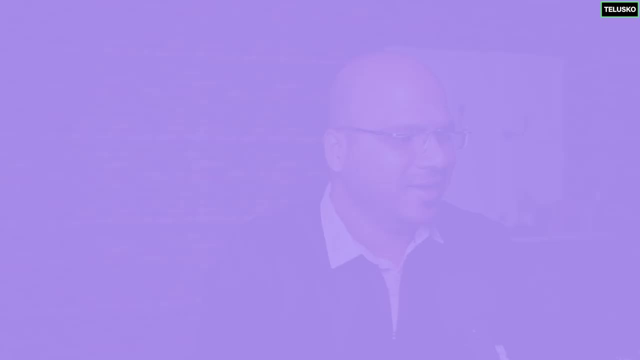 but you do. we create classes. how do we create object of those classes that we'll see in the next video.